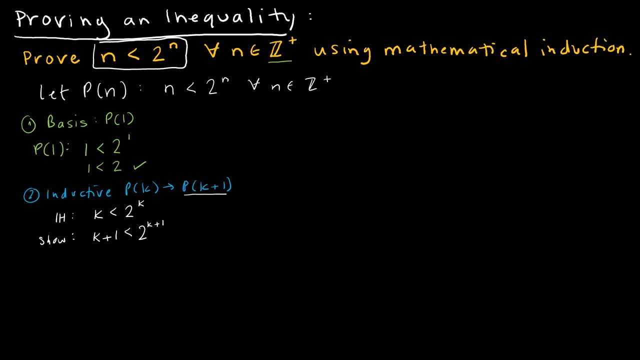 that's what I have for what I'm trying to show and what I can say is true, which is my inductive hypothesis. So now I'm going to go back to my inductive hypothesis. K is less than 2 to the k And I'm going to do whatever I need to do to make the left side 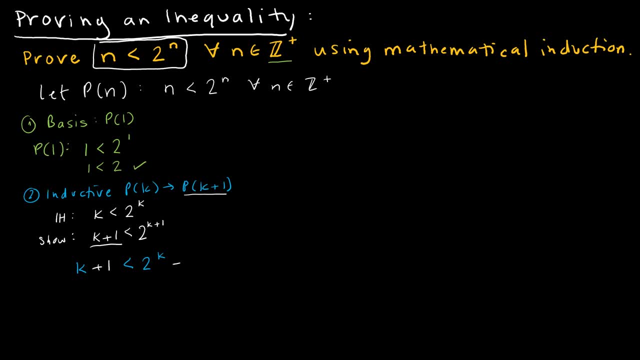 match what I want to show, So I'm just going to add 1 to each side. Now here's the tricky part, And this is the part you're either going to love or you're going to hate with a fiery passion. Most people hate it with a fiery passion Because it's 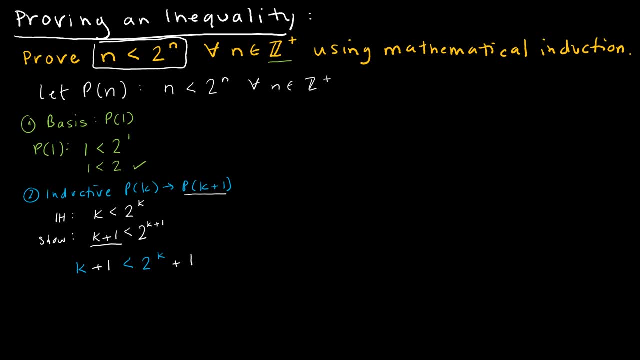 an inequality. we're not bound by the same rules of an equation. They don't have to be equal to one another. If I replace something in an equation, whatever I replace has to be equal to what I've replaced. If I replace something in an inequality, all I'm going. 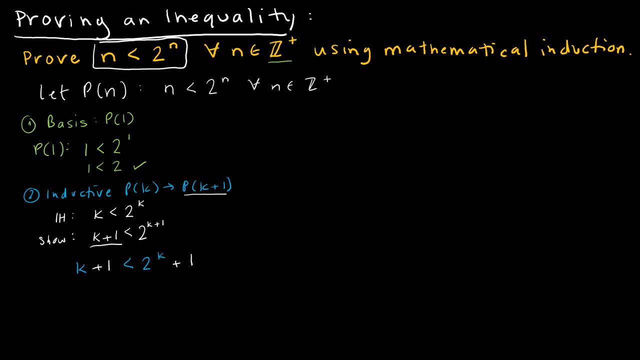 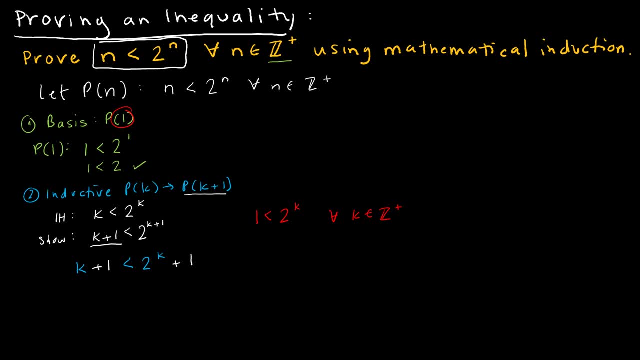 And I'm going to go back to my inductive hypothesis. So I know that going to get bigger and bigger and bigger. So I know that this is true. So what I'm going to do is I'm going to say, well, that is less than 2 to the k, And then, instead of 1,. 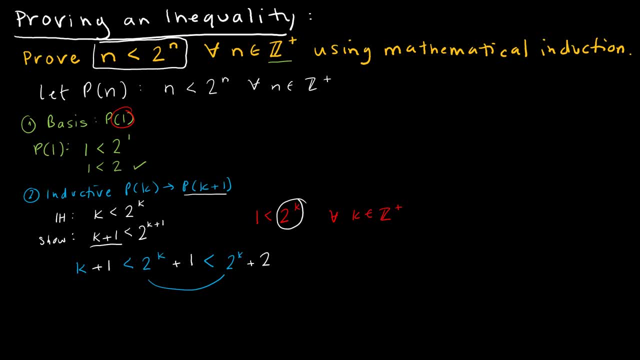 I'm going to replace it with 2 to the k. Now how can I do that? Because 1 is less than 2 to the k. So it's okay for me to do that, because I'm not breaking any mathematical law. I'm replacing 1 with something that's greater than that. 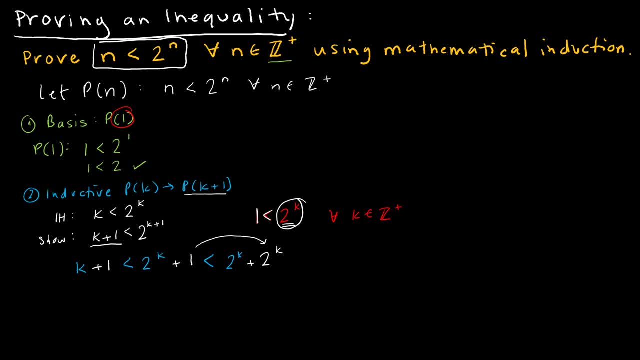 and saying, hey, this inequality still holds. So again. you might be thinking that's totally cheating, but this is how a proof by inequality works is now I've got k plus 1 on this side, and on the right side I have 2k plus 2k, which is essentially 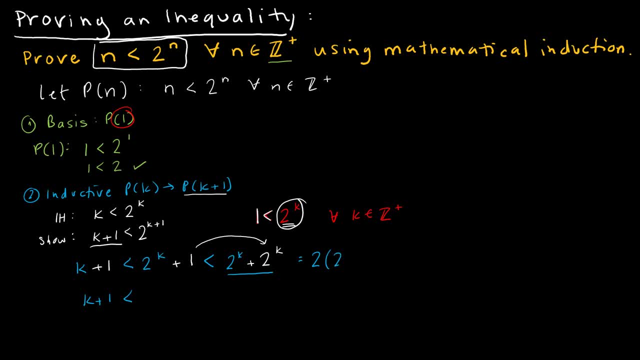 2- 2k's, which is, can you guess, 2 to the k plus 1.. So again, you might be really upset right now and think, well, where did she even come up with that? And again, it's just a matter of practice. 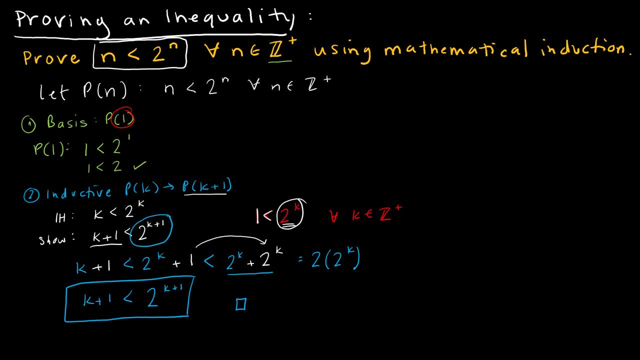 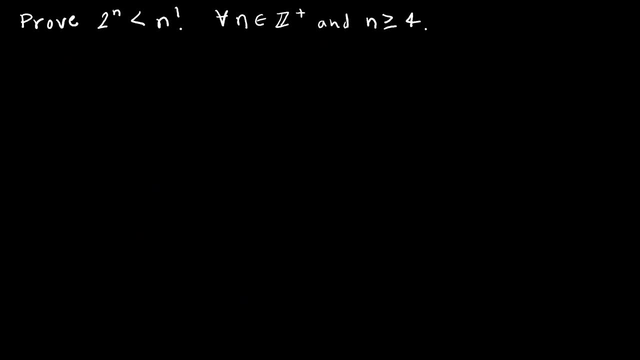 and again. that's where this comes in. I want to know where I'm headed, so I know what kind of math magic I need to pull to make this thing work. Let's see, Let's look at one more proof of an inequality, and again, you may hate these. 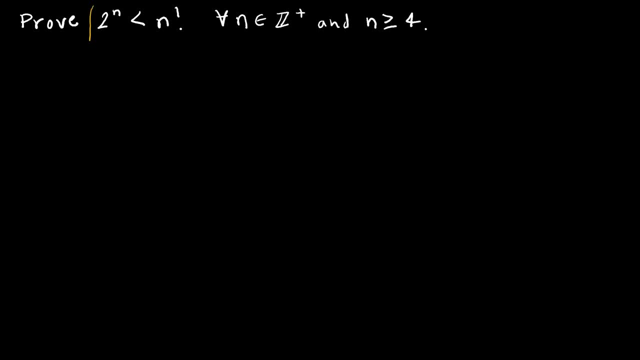 and I totally understand. but this one we're trying to prove that 2 to the n is less than n, factorial for all n's that are integers and greater than or equal to 4.. So that's going to come into play when I do my basis step, because of course my lowest or least value is 4.. 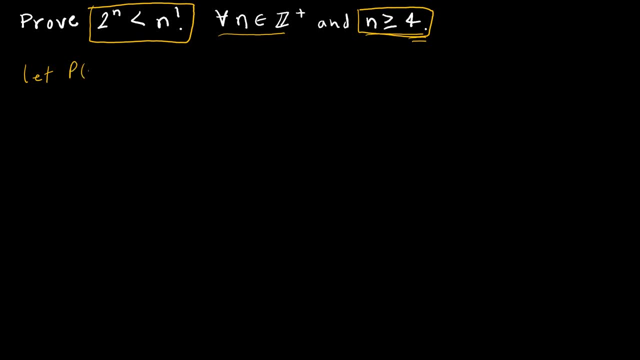 So I'm going to start by saying: let p of n represent that 2 to the n is less than or equal to the n is less than n factorial. Then I'm going to do my basis step, and my basis step is that the least value is true. So in this case that's p of 4.. So 2 to the 4th. 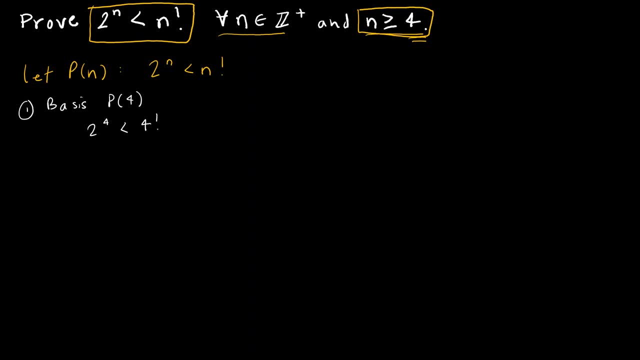 is that less than 4 factorial 2 to the 4th is 16.. Remember, 4 factorial is 4 times 3 times 2 times 1, which is 24.. So is 16 less than 24? Yes, it is. 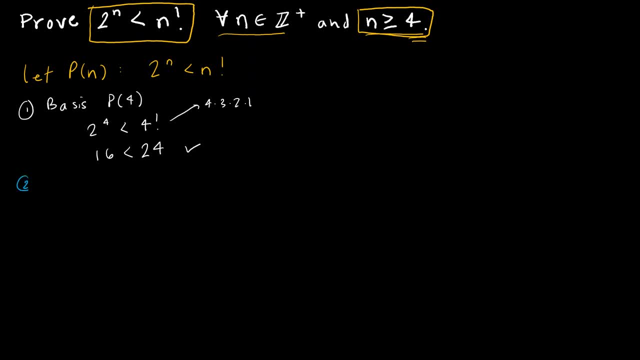 Then I'm going to do my inductive step And for my inductive step, recall that I'm going to assume pk and show that it implies p of k plus 1.. So we'll start with my inductive hypothesis, which is: whatever p of n is. 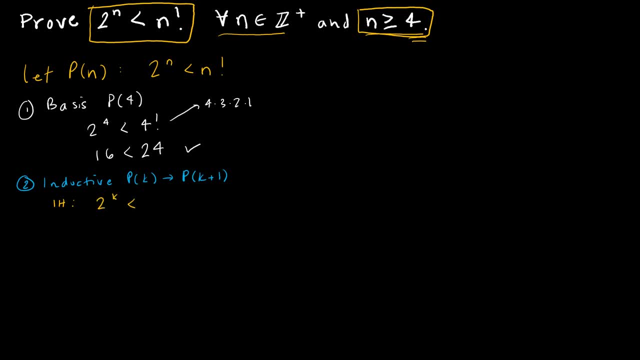 but which is 2 to the n is less than or equal to 4.. So let's do my inductive step: the k instead. so 2 to the k is less than k factorial. and what do I want to show? I want to show that I can replace k with k plus 1, and that still holds. so how do I? 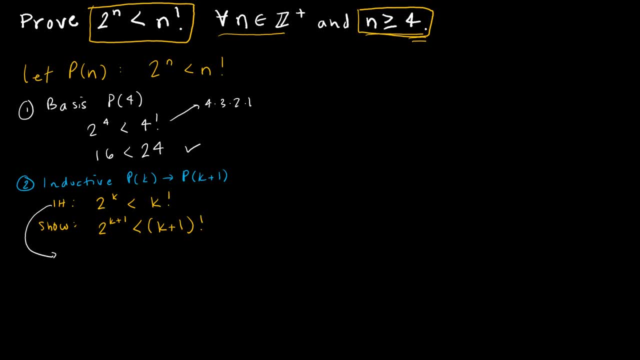 do that. I start with my inductive hypothesis: 2 to the k is less than k factorial. now what am I going to do to each side? remember that typically what I'm doing is I'm doing whatever I can to the left side of the equation to make it. 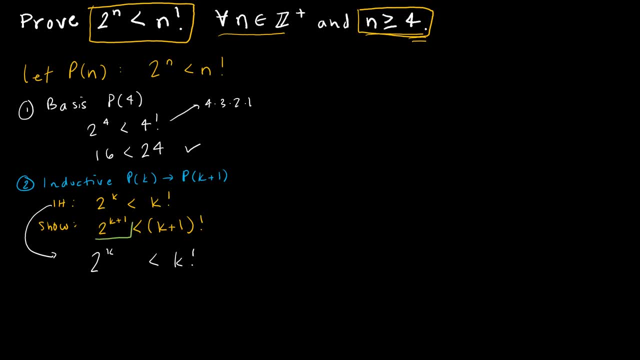 look like what I want to show. I'm trying to get to 2 to the k plus 1, so I'm actually going to multiply by 2 on each side. so hopefully we recall with our rules of exponents that if I have 2 to the first and I have 2 to the k, because 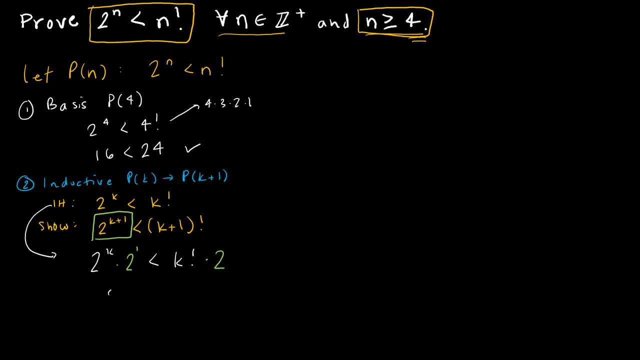 I have the same base. the left side now becomes 2 to the k plus 1. I can just add those exponents. now, on the right side, I have k fact. well, I have 2 times k factorial, 2 k factorial, which is okay, but keep in mind what I'm trying to get to. I'm trying to 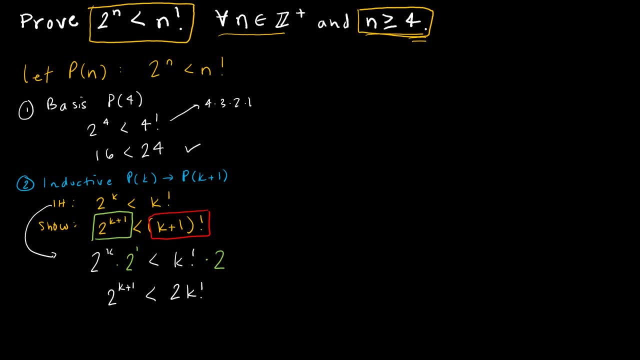 get to k plus 1 factorial. so again, this is the part that drives a lot of people crazy- is the only rule is I have to preserve the inequality. so if I can replace 2 with something greater than 2, then I'm okay, as long as 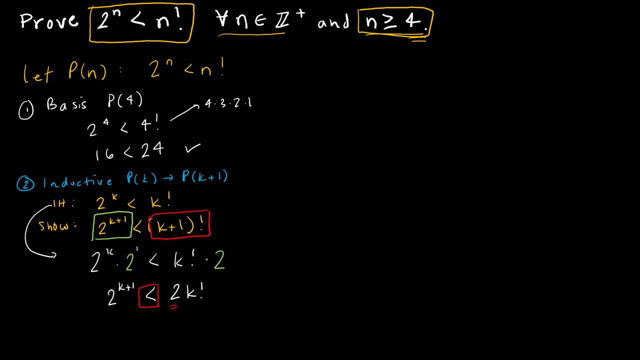 that's not less than 2. that would be breaking the law, mathematical law. so what I'm going to look at is: where am I trying to get to? I'm trying to get to k plus 1 factorial. so can I say that 2 is less than k plus? 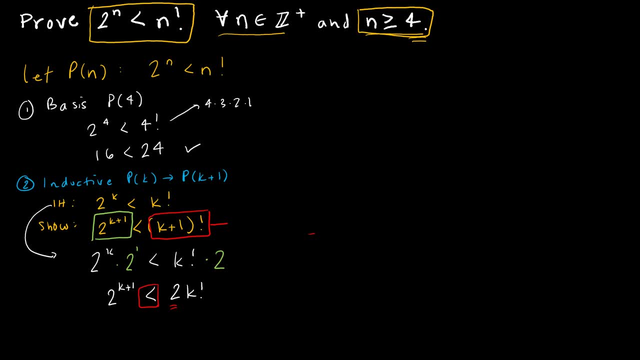 1, or maybe it would make more sense to you to say that k plus 1 is is greater than 2.. Now, why do I want that to be? Well, I need to replace 2 with something greater than 2.. And I'm going to use k plus 1.. And do you believe me that k plus 1 is greater?